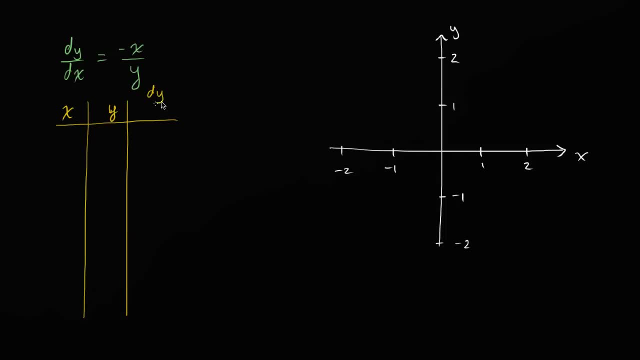 So x, y and this is dy dx. So let's say: when x is zero and y is one, what is the derivative of y with respect to x? It's going to be negative zero over one, so it's just going to be zero. 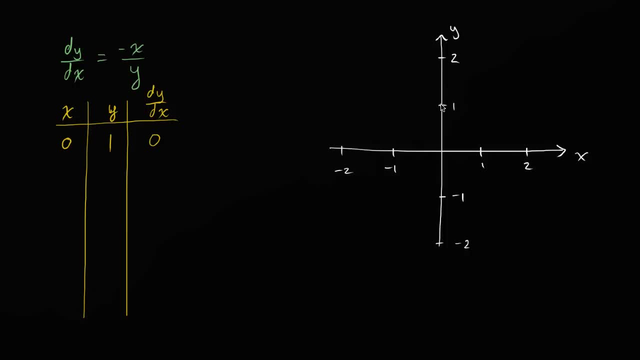 And so at the point zero one, if a solution goes through this point, its slope is going to be it's going to be zero, and so we can visualize that by doing a little horizontal line segment right there. So let's keep going. 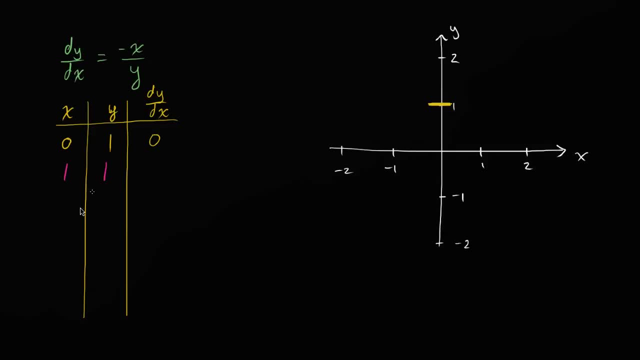 What about when x is one and y is one? Well then, dy dx, the derivative of y with respect to x, is negative one over one. So it's going to be negative one. So at the point one comma one, if a solution goes through that point. 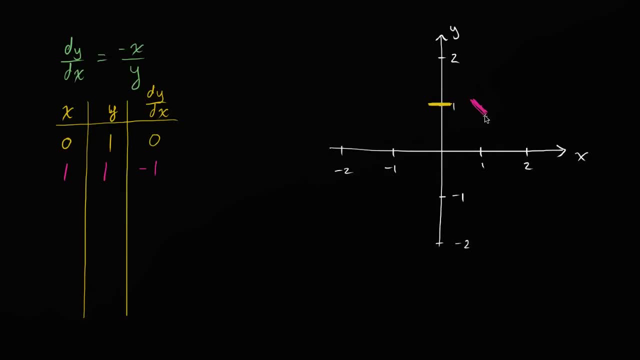 it would have a slope. it would have a slope of negative one, And so I draw a little line segment that has a slope of negative one. What about when x is? let me do this in a new color. what about when x is one and y is zero? 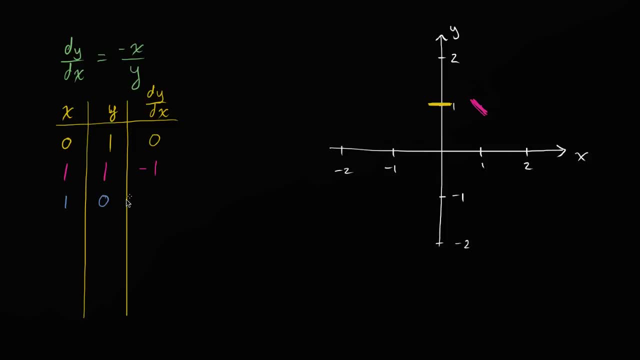 Well then it's negative, one over zero. So this is actually undefined, But it's a clue that maybe maybe the slope there, I guess, or if you had a tangent line at that point, maybe it's vertical. So I'll put that as a question mark: vertical. 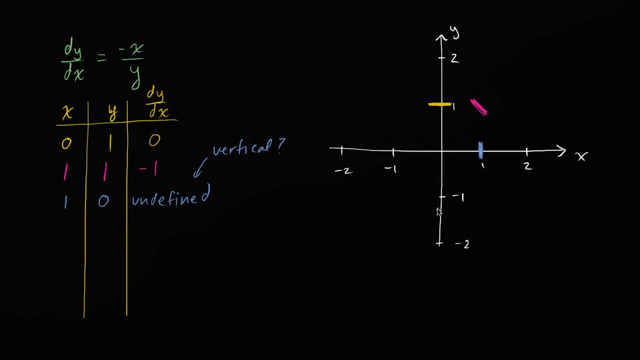 There, And so maybe it's something like that. if you actually did have, I guess it wouldn't be a function if you had some kind of relation that went through it. But let's just put, let's not draw that just yet, but let's try some other points. 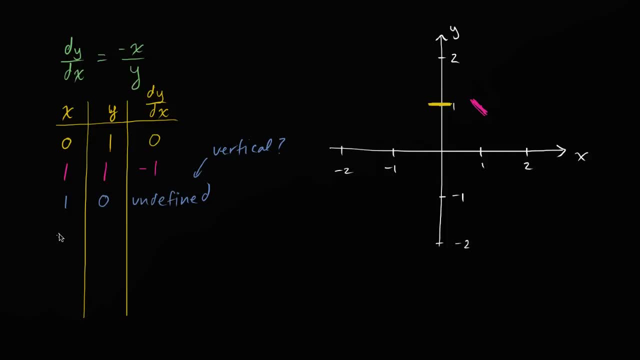 Let's say that we had- let's try the point- negative one, negative one. So now we have negative, negative one, which is one over negative one. Well, you would have a slope of negative one here. So negative one, negative one. 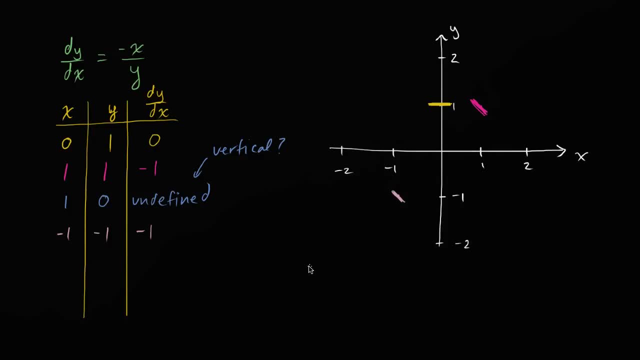 You would have a slope of, you would have a slope of negative one. What about if you had one negative one? Well, now it's negative one over negative one. Your slope is now one. So one negative one. If your solution, if a solution goes through this, 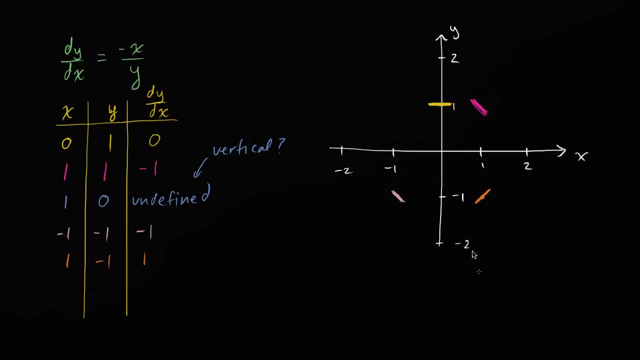 its slope would look like that And we could keep going. We could even do two negative two. That's going to have a slope of one as well, If you did- if you did- positive two, positive two, that'd be negative, two over two. 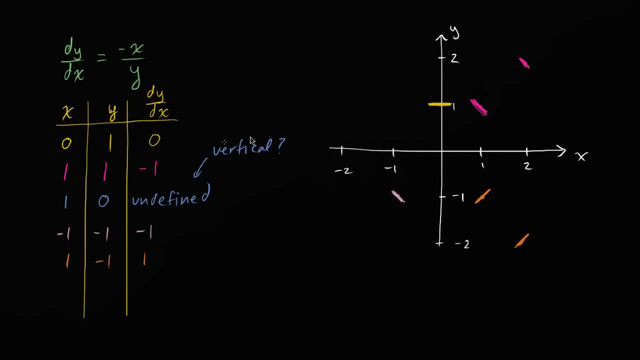 You'd have a slope of negative one right over here, And so we could do a bunch of, we could do a bunch of points. Just keep going. I've now, I'm now just doing them in my head, I'm not going on the table. 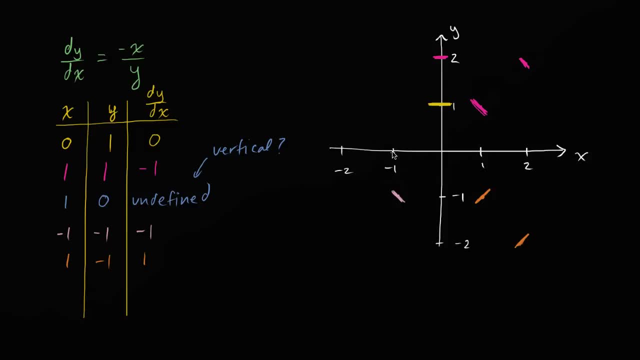 But you get a sense of what's going on here. Here your slope would: if it was negative one one, It's going to have a slope of one. So at this point your slope: negative one one. So negative negative one is one over one. 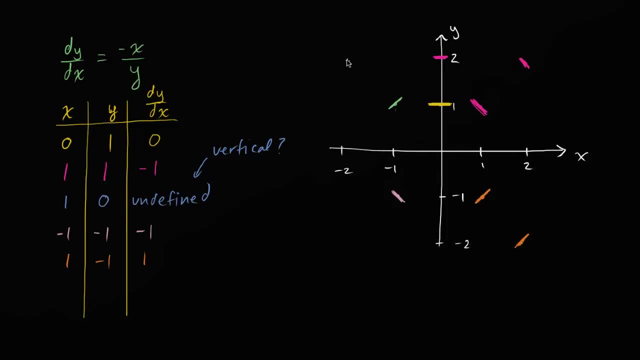 So you're going to have a slope like that And negative two, two. Same exact idea. it would look like that, And so you get a when you keep drawing these line segments over at these kind of these sample points in the Cartesian or in the in the XY plane. 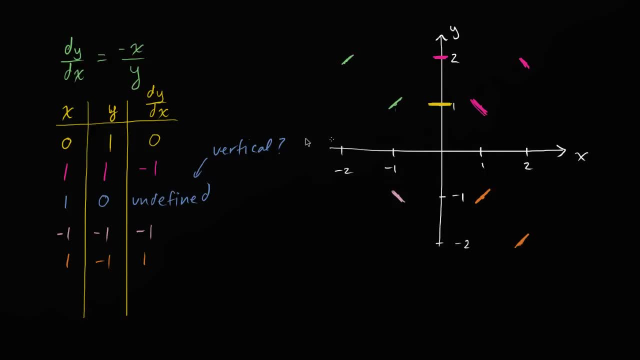 you start to get a sense of, well, what would a solution have to do? And you can start to visualize that, hey, maybe a solution, a solution would have to do something, something like this: This would be a a solution. 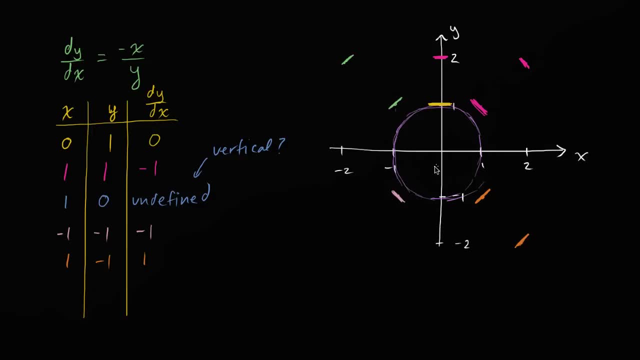 So maybe it would have to do something like this. Or if we're looking, if we're looking only at functions and not relations- you know, I'll only I'll make it, so it's a very clear- So maybe we would have to do something like this. 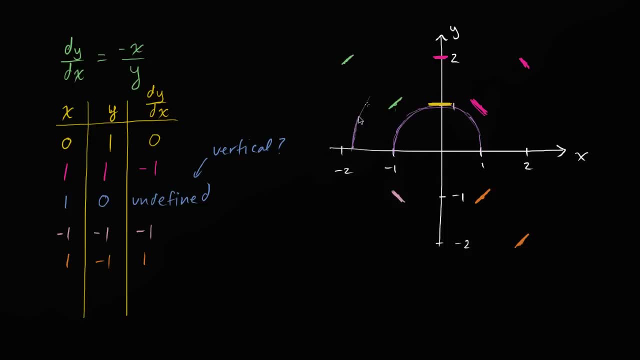 Or if a if the function started like here, based on what we've seen so far, maybe we would have to do something. maybe we would have to do something like this, Or if it was, if this were a point on the function over here. 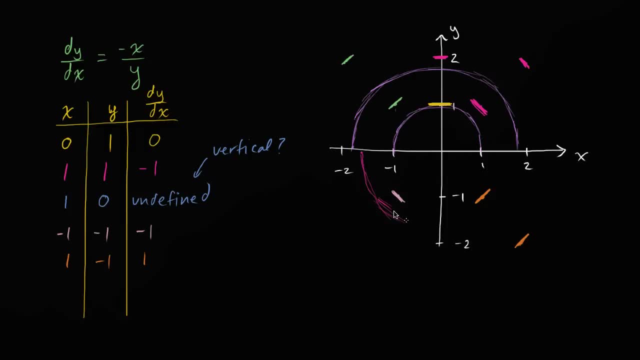 it would have to do something like this. And, once again, I'm doing this based on what the slope field is telling me. So this field that I'm creating, where I'm taking, I'm sampling a bunch of points and I'm visualizing the slope with the line segment. 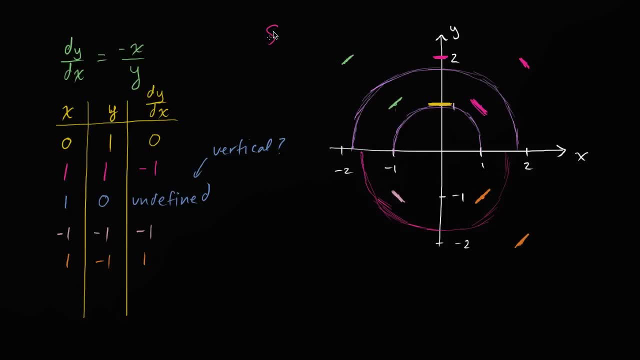 once again, this is called a slope slope field, So hopefully that gives you kind of the basic idea of what a slope field is. In the next few videos we'll explore this idea even deeper.